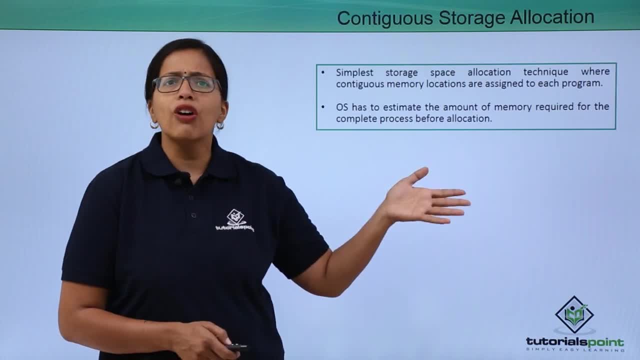 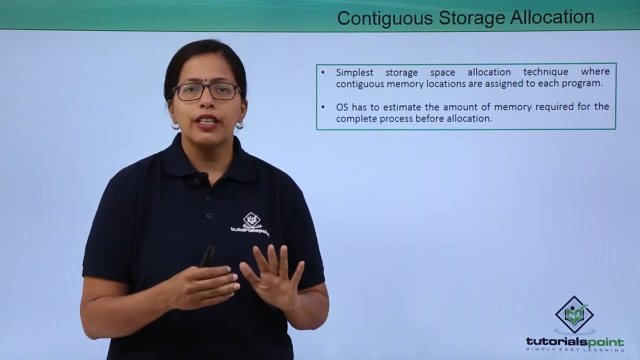 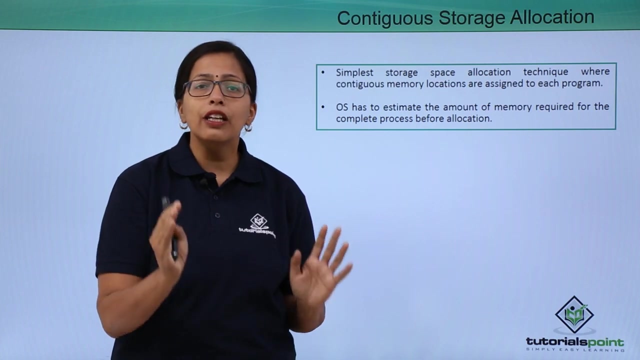 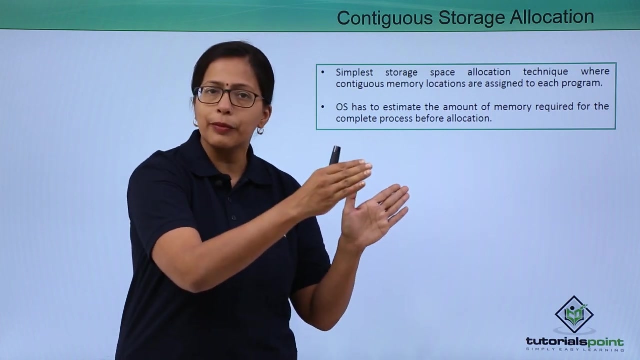 it is. Let's see what these techniques are. The first and the foremost, or the easiest one, is contiguous storage allocation. Contiguous means continuous. What the operating system will do the moment the job comes. it will make an estimate of how much memory is required and it will allocate that chunk of memory in the secondary memory as well as the primary memory, The amount that is required in the primary memory and the amount that is required in the secondary memory. However, this has 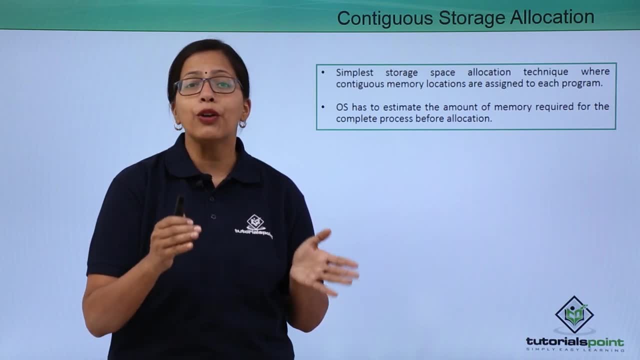 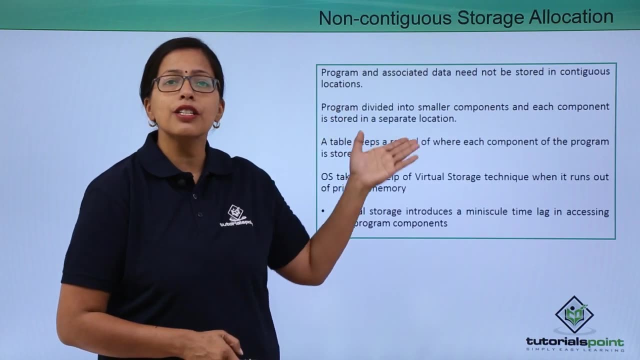 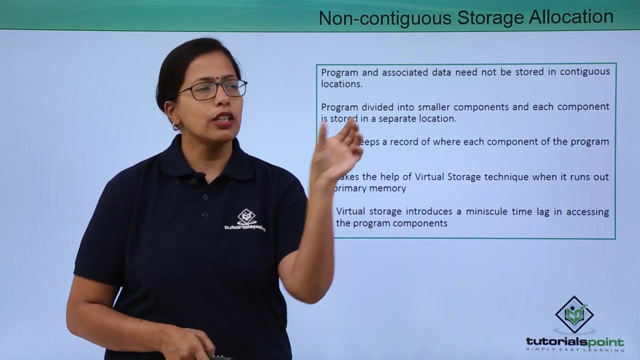 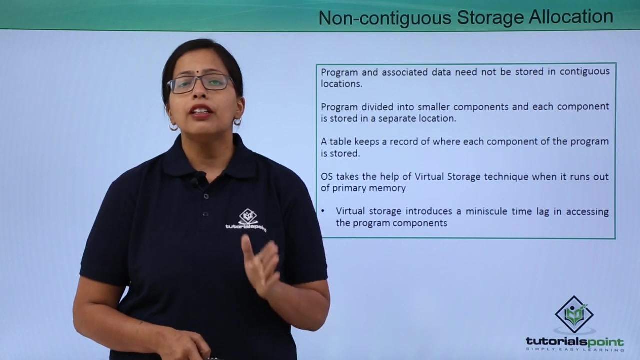 a small problem: That whole chunk might not be available. So in reality, the operating system will use a non-contiguous storage allocation technique. What does that mean? Non-contiguous? that means non-continuous. So there is one chunk that is available here. There is one chunk of memory that is available here. There is one chunk of memory available here. So what the operating system will do, it will break down the program or the job into different parts. 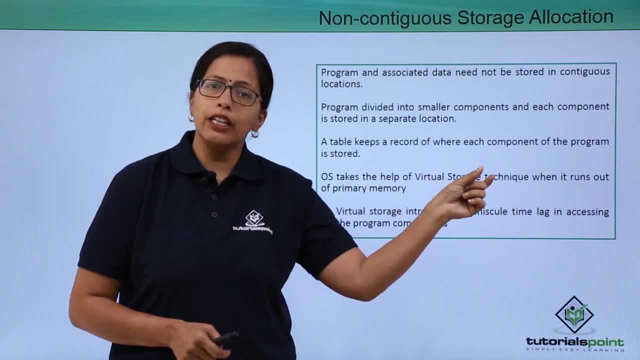 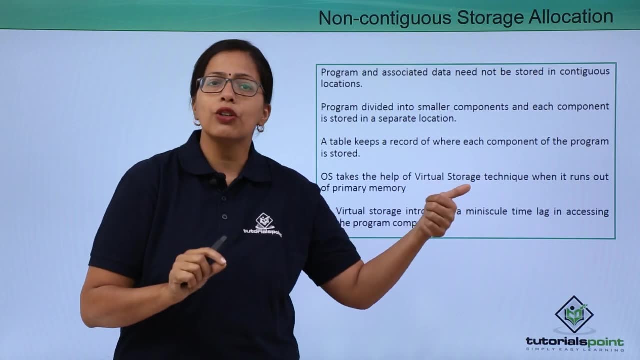 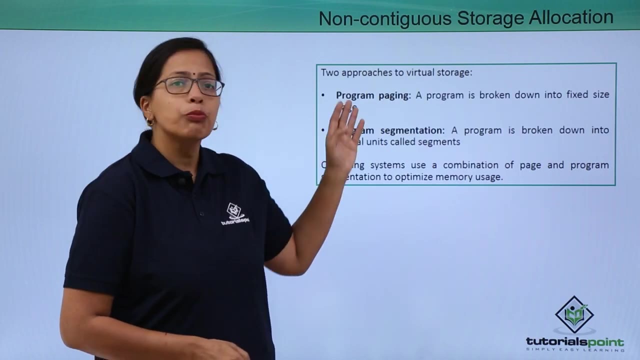 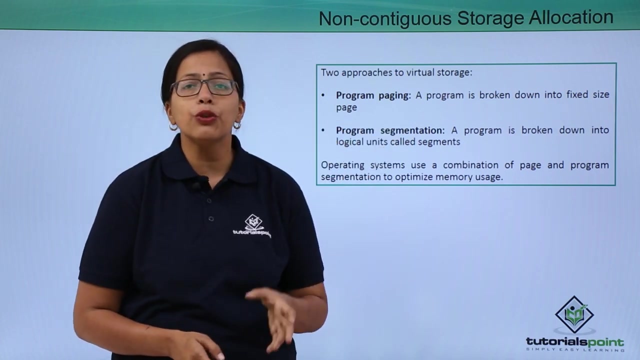 Different segments and each segment will be stored in one location. It will have a table where the address, the memory address of the starting location will be stored. Now how this breaking down is done. It is done in two ways: Program paging and program segmentation. What happens in program paging? A program is broken down into fixed size page. Say operating system has already decided. 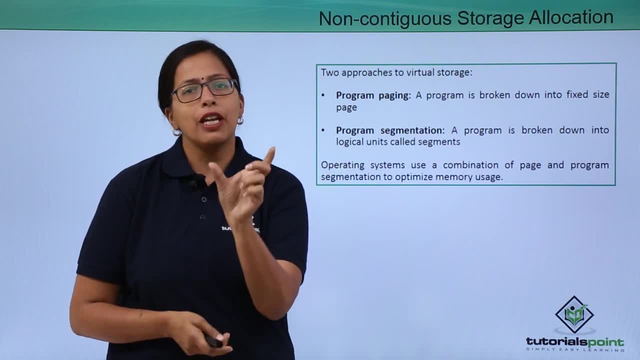 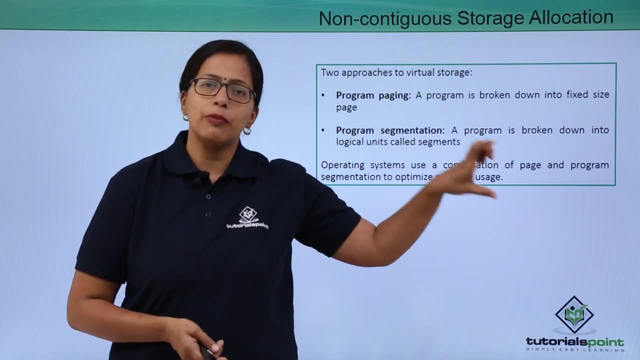 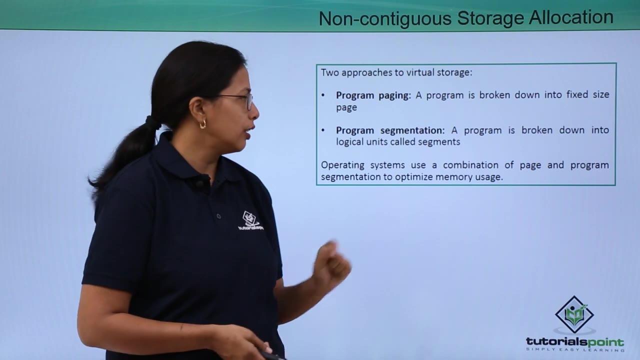 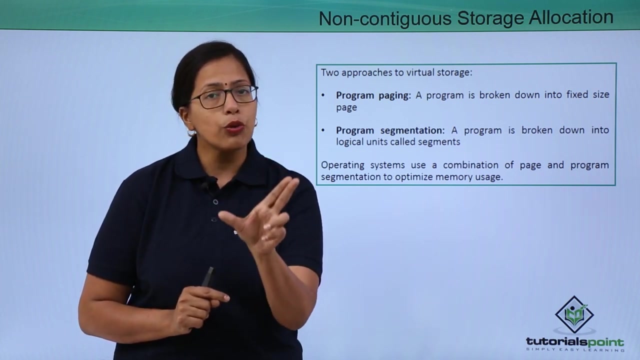 that it will have 8 bytes of page length. So it will divide the program that has come into 8 bytes. 8 bytes, 8 bytes. Okay, One 8 byte will be stored in one location. One 8 byte will be stored in one location. So that is what program paging does. There is another method: Program segmentation. Here the program is not broken down into fixed memory lengths, but they are broken down logically. Say one program segment or one part of the program is doing one function. So